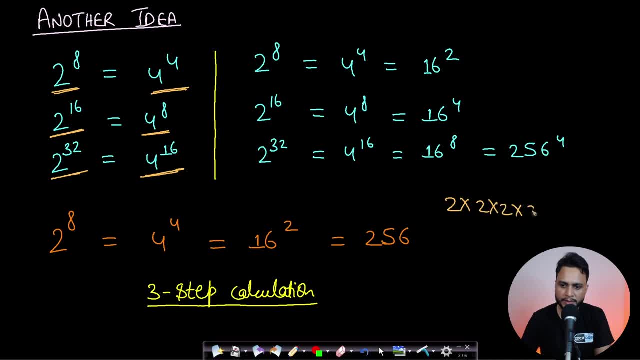 you see, let's say I write two four times. right, If I write two four times, it is equivalent to two to the power four. Now two to the power four. I'm saying that it can also be written as four to the power two. And how is this happening? Let's say we club this two twos together. Now you can write them as four and this will become another four. Now, if you multiply them, then it will turn out to be four to the power two. So with this logic we can say that two to the power eight can also be written as: 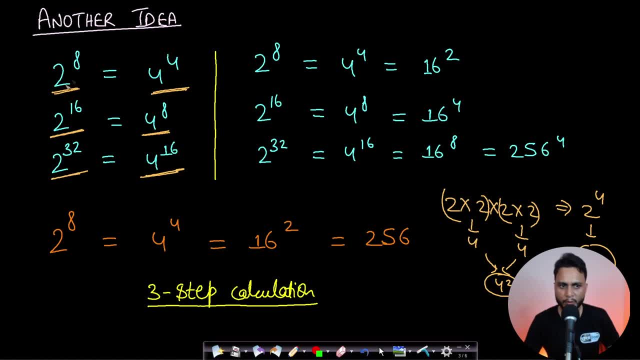 four to the power four. This is nothing but squaring the base and taking half of the exponent, And this is pretty logical. This is a very simple example for the same logic. Now, using the same logic, we can also say that two to the power eight can be written as just square the base and half. 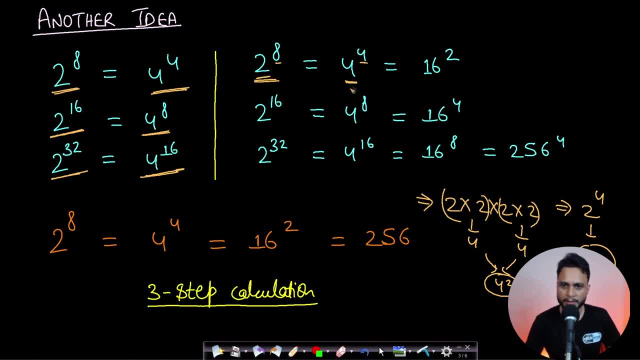 the exponent And you can write it as four to the power four And simply four to the power. four can be written as just square, the base and half the exponent. So four square will be 16 and half of this four will be two. So 16 to the power two, right Even again, if you start extending it. 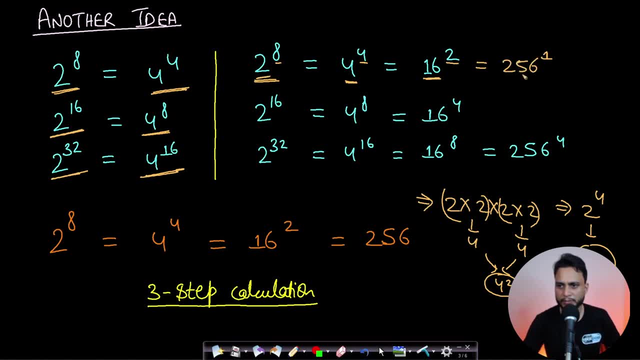 it will be 16 square, which is, I think, 256 to the power one. So you will see that two to the power eight. final answer is 256.. Instead of following this technique, if you had followed the previous technique of the simple approach of like multiplying two eight times, then that would. 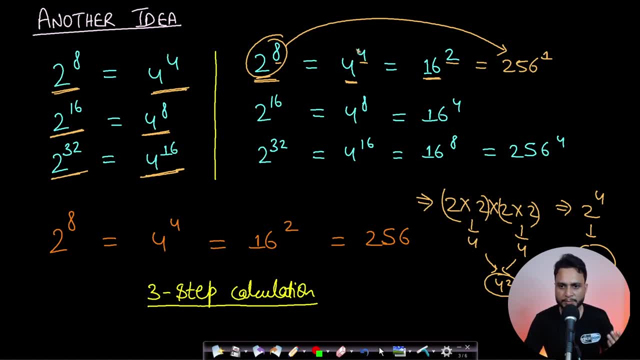 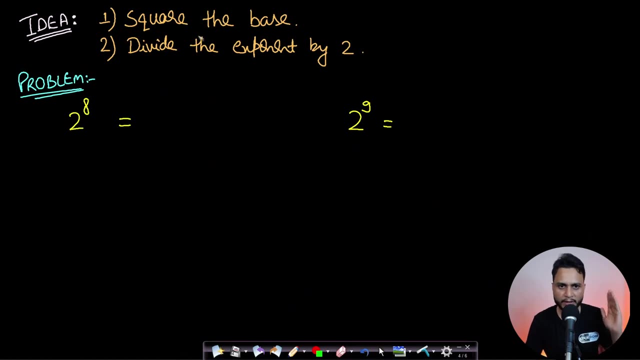 have given you 256, but in eight number of steps. In this case you see that there are only three steps: one, two and three, right? So this is heavily reducing the number of steps. So let's solve an example with this idea. Now, if you look at the idea, it is just squaring the base and 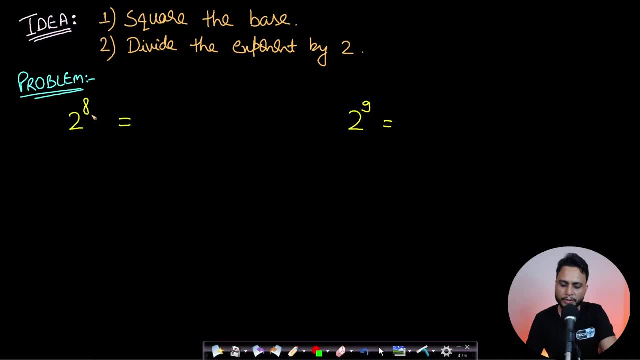 dividing the exponent by two. So let's take two to the power eight. So if we take two to the power eight, then we can write it as two to the power four into two to the power four, which is like dividing it into two parts, And simply this can be written as four to the power of four. Okay, 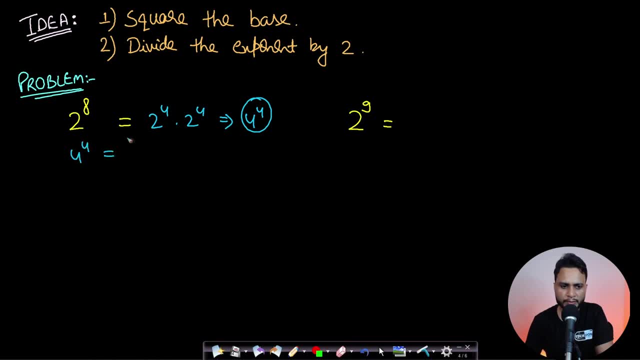 now, if we take again four to the power four, we can write it as 16 to the power of two. with the same logic, And again, if we take 16 to the power two, we can write it as 256 to the power one. And 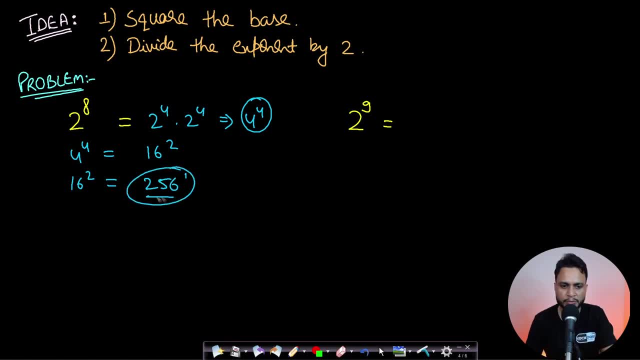 whenever you reach to power one, that is where you stop. So 256 is your final answer for two to the power eight. Now, if you try solving a similar problem, two to the power nine, where the power is odd, you will definitely fall into a problem Like if you divide this nine by two. 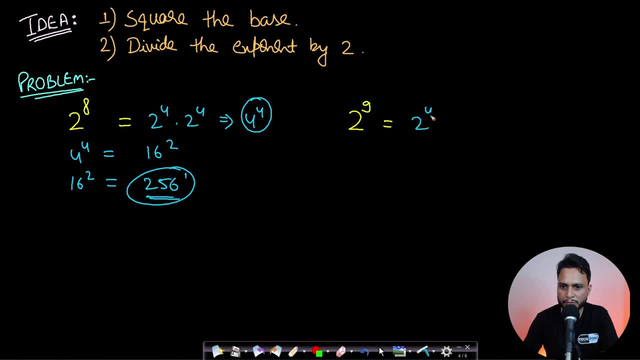 it will be four, right. So you have to write it as two to the power four into two to the power four, into two to the power one. So you will see that this two to the power one is not matching this two to the power four, And this is just an extra value which is equal to the base. So this has to. 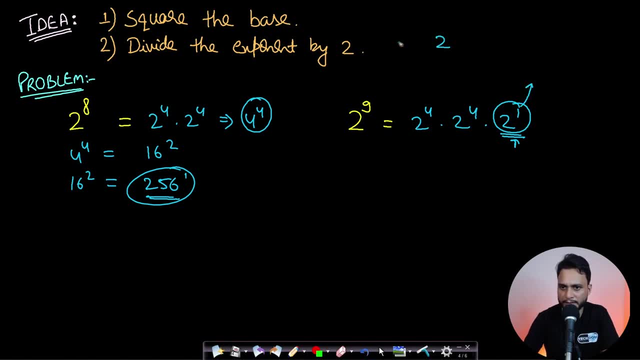 be saved somewhere. So let's save to two to the power one, somewhere, right, And let's call it result. Now, once we get two to the power four, like this can be written as four to the power of two: right Now, this four to the power four can be again written as 16 to the power two, And again. 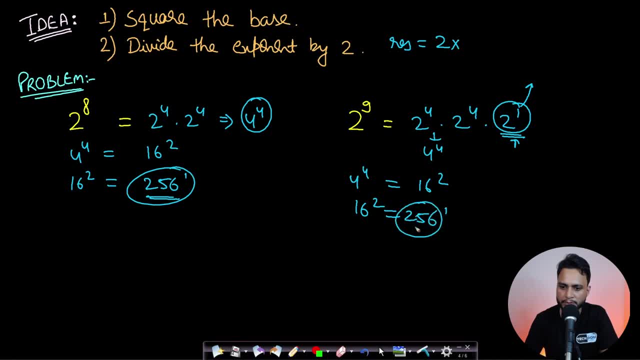 16 to the power two will become 256 to the power one. So you will see that 256 is the final answer here And there was something which was lost due to dividing an odd number by two, And hence it was saved in result. So, finally, this 256 will be multiplied by this result And it will become 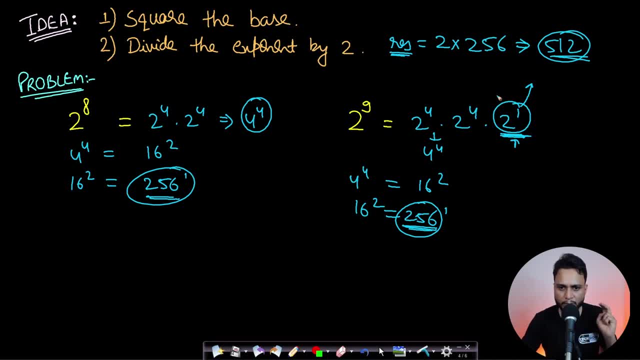 five, one, two. So you will see that there is only one, two, three, four, five, four, five, five. one thing you need to take care of in case of the odd powers, for even powers dividing by two. 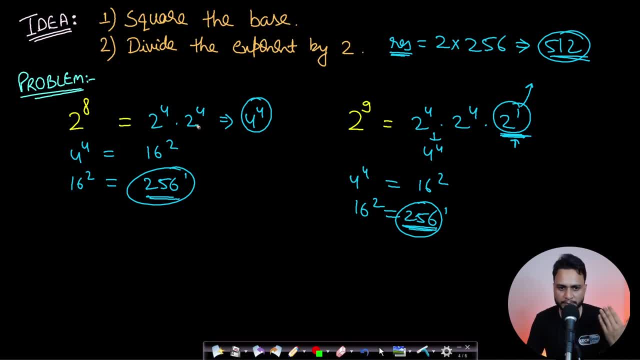 actually doesn't make you lose any power, like any of the base value, And when the odd number comes, like when the power is odd, then you will definitely lose one of the values. Okay, so that has to be saved somewhere, And that is where the result actually comes into picture. 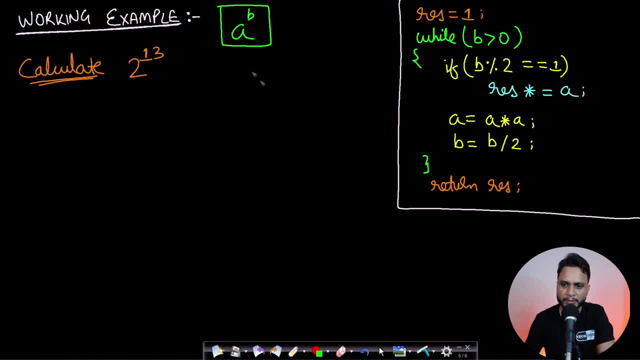 So let's take one of the problem and do a dry run of the entire logic And you will easily understand. So the right hand side is actually the entire code of the logic which we discussed, which is binary exponentiation, And on the left hand side, let's take an example. 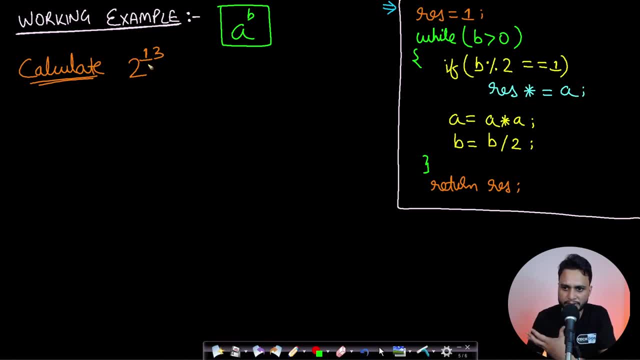 two to the power 13.. And, by the way, this technique is known as binary exponentiation: binary because we are dividing by two, and exponentiation because the base is exponentially increasing and the steps are reduced to logarithmic order. right, So let's just do. 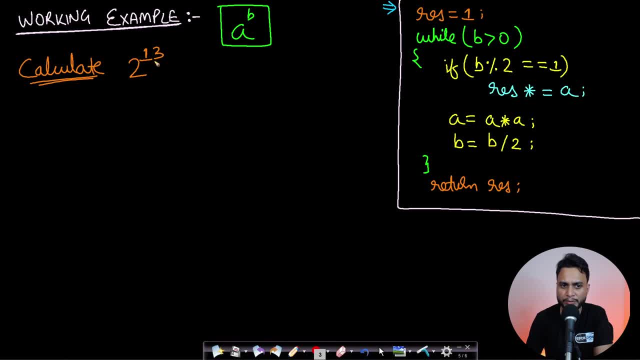 a dry run on this entire code. So let's take the example of solving two to the power 13.. So if you take two to the power 13, and let's also take all the variables, So the variables are result, which is equals to one, and then you have a and b, So a is equals to two and b is equals to 13,. 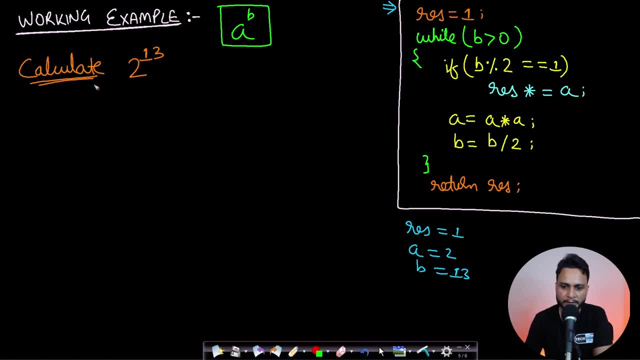 right, which is a to the power b format. Now, in the first step you will see if b is greater than zero. So two to the power 13.. Again, it can be written as two to the power six, two to the power six into two to the power one. Now this has to be saved somewhere, So definitely. 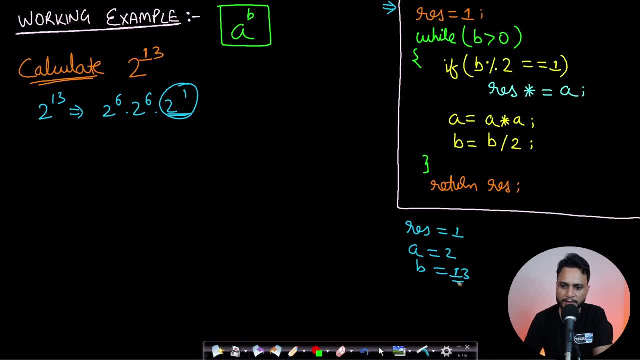 if b mod of two, where b is 13 in this case, right. So if b mod of two, that means if b is a odd number, then definitely this two to the power. one has to be saved in the result. So this result will. 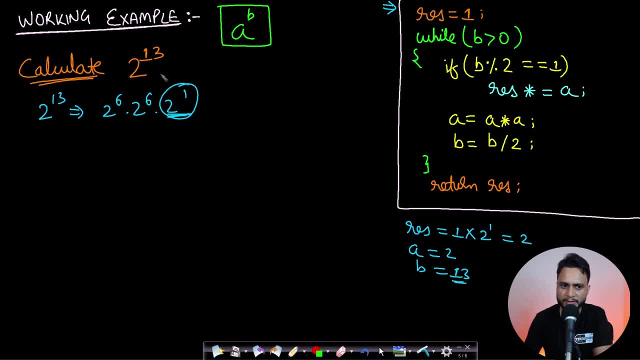 be multiplying to the power one, and this will become two. And in the next step you square the base, So the base will become four and the exponent will be halved. So now the next problem to be solved is four to the power six. Now, is this six an odd number? you will see that no. 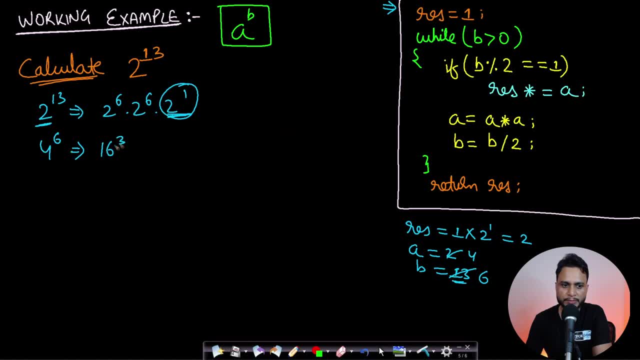 it is not an odd number. So definitely you can write here 16 to the power three for this. So what we are basically doing is just squaring the base and making the exponent go to half. So now you have a problem. 16 to the power three. So we can write 16 to the power three as 16 to the power. 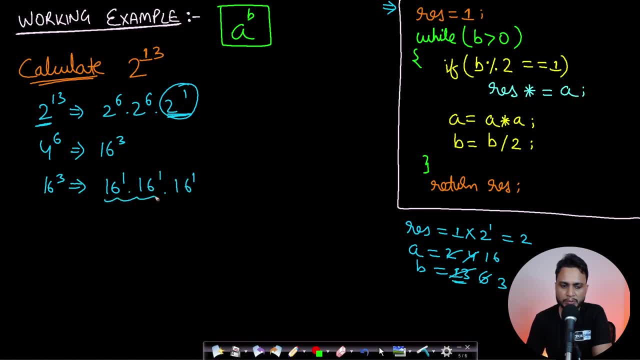 one into 16 to the power, one into 16 to the power one. Now these two can be clubbed together And it can be written as 256 to the power one. Okay, And this is an extra value because the power was an. 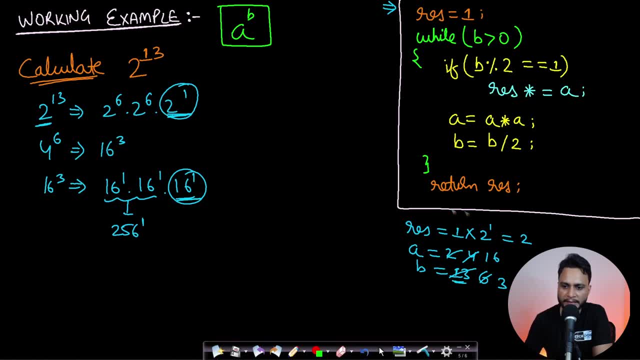 odd number. Now this has to be saved somewhere and and that will be saved in the result. So you will be multiplying 16 to the power one here, And this will make it 32.. Right, And now you have 256 to the power one. you will see that again, B greater than zero is true, And you will see that the power 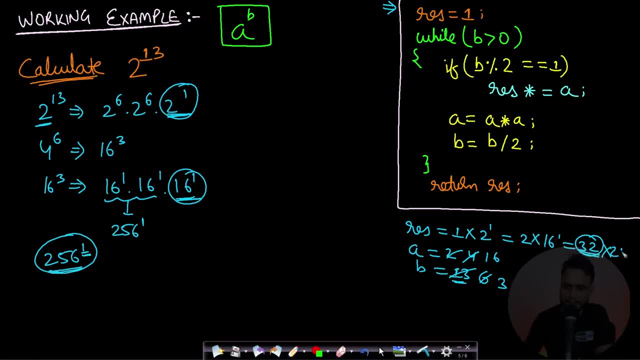 one is odd, So this 256 has to be multiplied here. This will be present at this place And you will get the final result as 8192.. And again, in the next step, this 256 will be squared up and this one will be halved. So one by two will become zero.